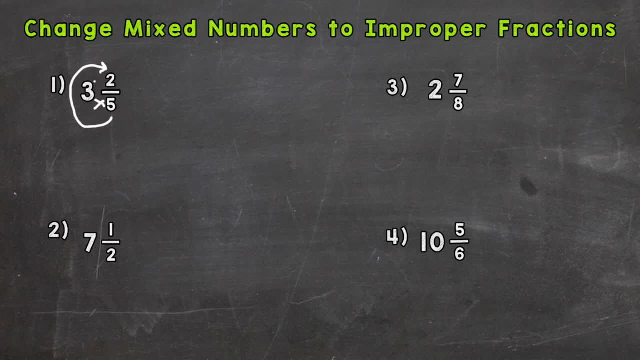 the five times the whole number and then add the numerator. So we would do five times three plus two. So five times three is fifteen plus two is going to give us seventeen. That's going to be the numerator of our improper fraction, And then we just keep the denominator. 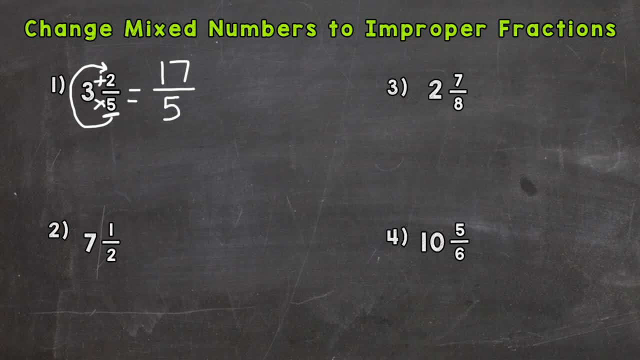 the five the same. And there we have it. There's our improper fraction. Now, three and two fifths is equivalent to seventeen fifths. So we're going to multiply that by five. So we're going to do five times three plus two. 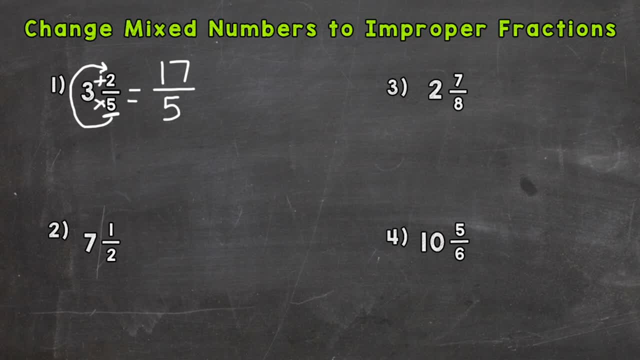 is equivalent to seventeen over five. Both of those, the mixed number and improper fraction, hold the same value. We just changed the form. Now we should be able to go back to a mixed number and get the same thing. And remember, to get back to a mixed number, we do seventeen divided by five. 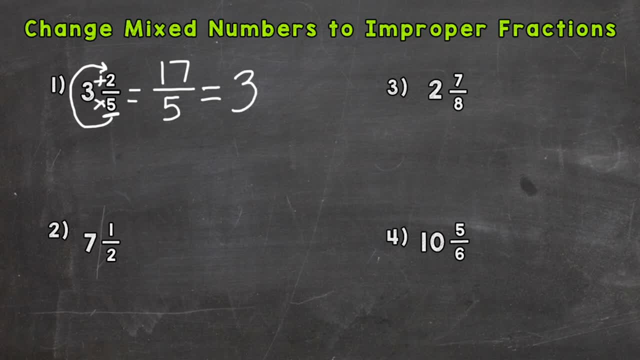 the numerator divided by the denominator. How many whole groups of five can we pull out of seventeen? It gets us to fifteen. So we have a remainder of two, two left over And we keep the denominator of five. So just to double check our answer, we went back to a mixed number and got the 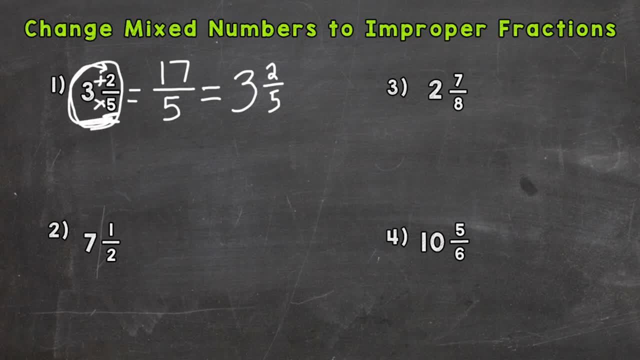 same thing that we started with, But the improper fraction for three and two fifths is seventeen fifths. So let's go to number two here. We're going to make our c here and start at the denominator and go to the top, And it's always multiply and then add, Always multiply, then add. 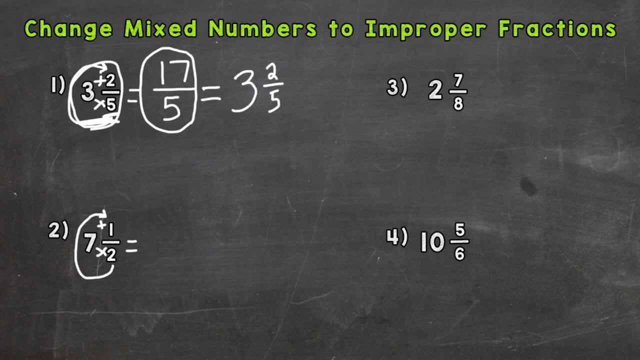 So the first thing we do: two times seven, which is fourteen plus that one, gives us fifteen, And we keep the denominator the same. So fifteen halves or fifteen over two would be our improper fraction. So let's hop over to number three. here, Let's make our c 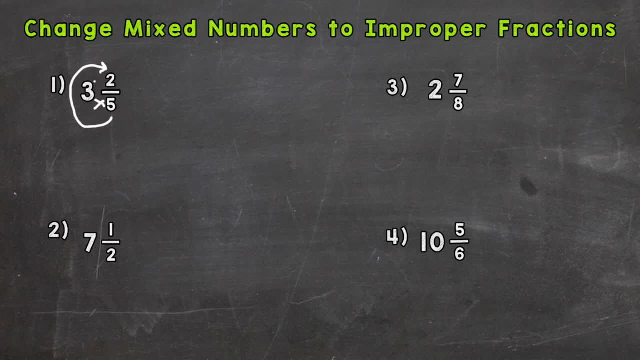 the five times the whole number and then add the numerator. So we would do five times three plus two. So five times three is fifteen plus two is going to give us seventeen. That's going to be the numerator of our improper fraction, And then we just keep the denominator. 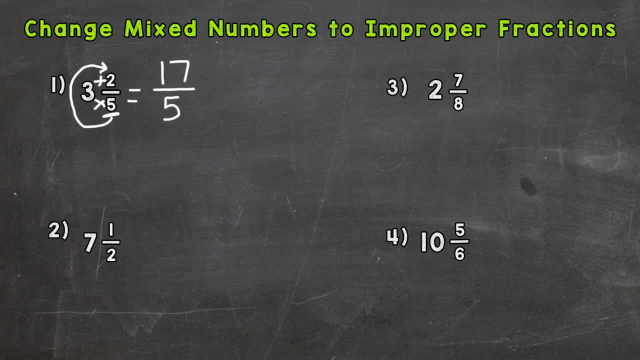 the five the same. And there we have it. There's our improper fraction Now. three and two fifths is equivalent to seventeen fifths. So we're going to multiply that by five and we're going to get seventeen over five. Both of those, the mixed number and improper fraction, hold the same value. We just change the. 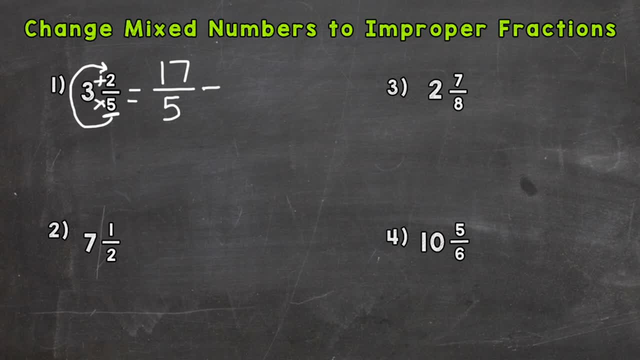 form. Now we should be able to go back to a mixed number and get the same thing. And remember to get back to a mixed number. we do seventeen divided by five, The numerator divided by the denominator. How many whole groups of five can we pull out of seventeen? Well, three whole groups. 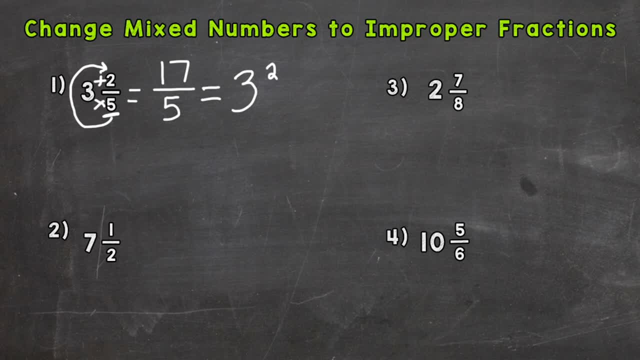 Fifteen. So we have a remainder of two, Two left over And we keep the denominator of five. So just to double check our answer, we went back to a mixed number and got the same thing that we started with, But the improper fraction for three and two fifths is seventeen fifths. 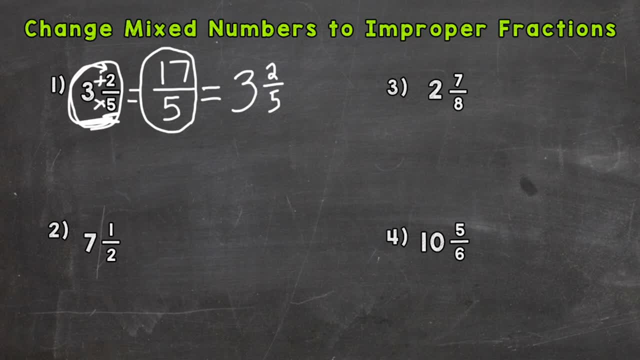 So let's go to number two here. We're going to make our c here and start at the bottom and go to the top, And it's always multiply and then add, Always multiply, then add. So the first thing we do: two times seven, which is fourteen plus that one, gives us fifteen. 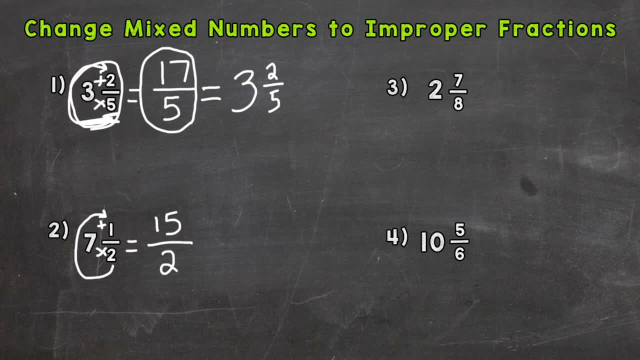 And we keep the denominator the same. So fifteen halves or fifteen over two would be our improper fraction. So let's hop over to number three. here Let's make our c. This always helps me remember that we start at the bottom. 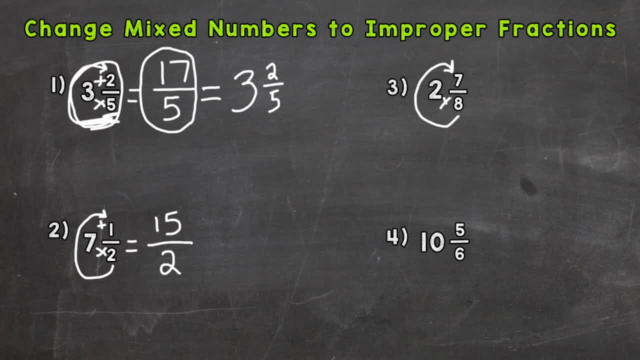 multiply and then add. So again multiplication, then addition: Eight times two is sixteen plus that seven gives us twenty three. And again we keep our denominator the same, which is eight be 23 eighths. And lastly, number 4- here start at the bottom, multiply and then add 6 times 10. 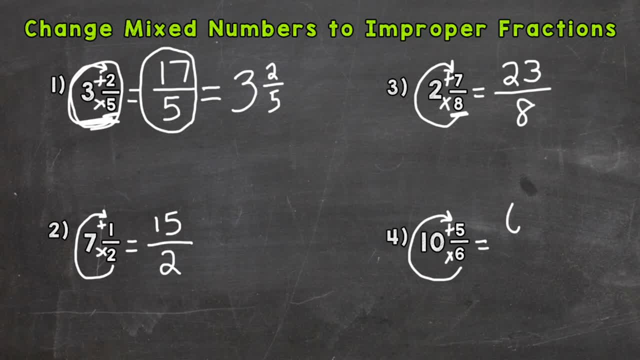 is 60,, plus that 5 is 65.. Keep the denominator the same: 65 sixths would be our improper fraction for number 4.. So there you have it. There's how you change mixed numbers to improper fractions. Hopefully that helped and gave you what you were looking for. Thanks so much for watching. Until next time, peace. 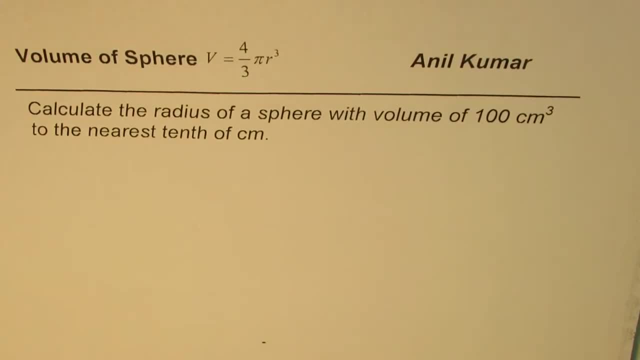 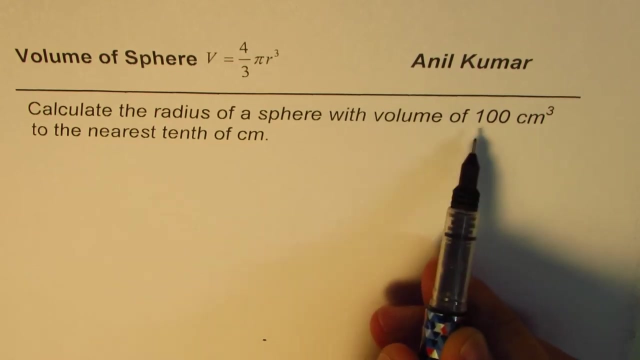 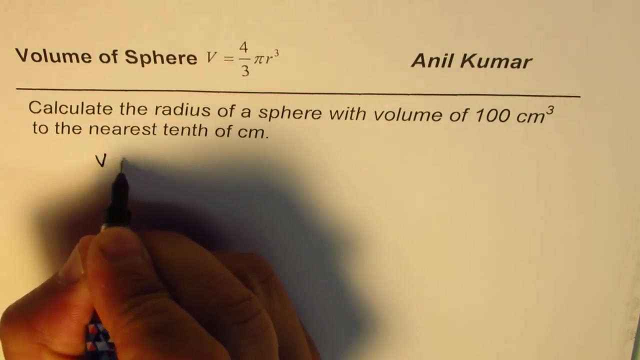 I'm Anil Kumar and in this video we'll learn a technique to find radius of a sphere when its volume is given to us. The question here is: calculate the radius of a sphere with volume of 100 centimeter cube to the nearest tenth of centimeter? Well, the formula for volume is volume. 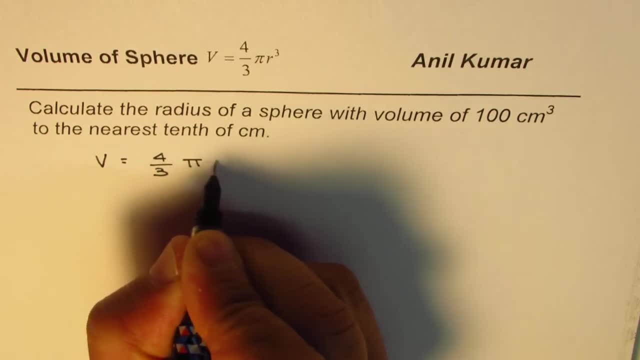 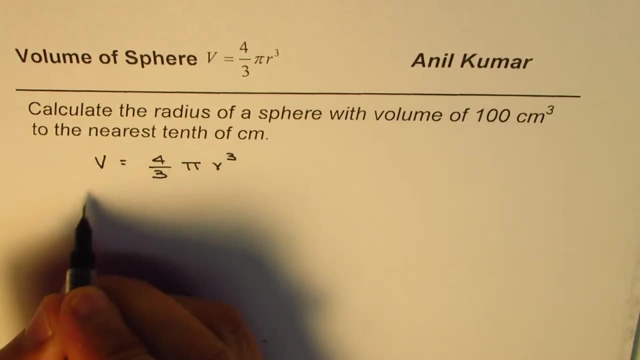 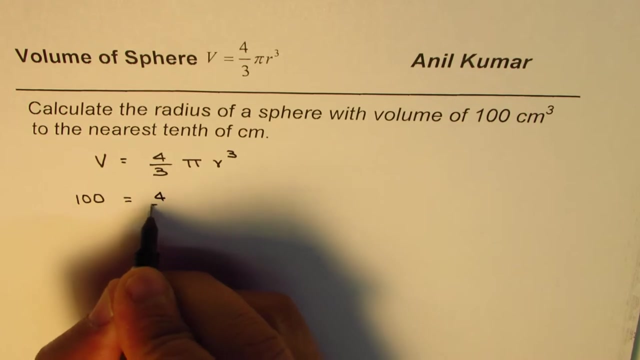 is 4 by 3 pi r cube. Now, in this particular case, we are given the volume, which is 100 centimeter cube, So write volume as 100 for the time being. Well, it includes units in the answer: 4 by 3 pi. 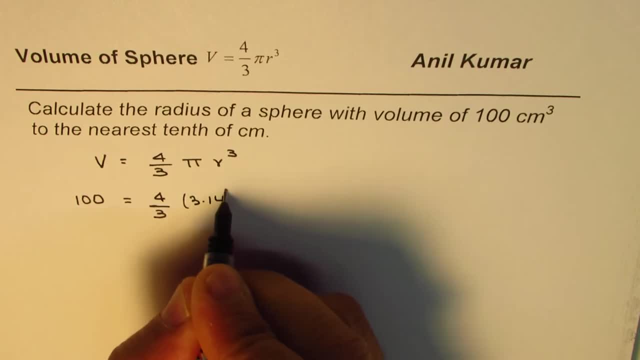 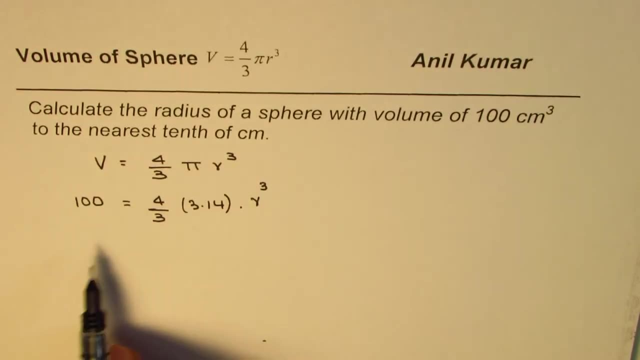 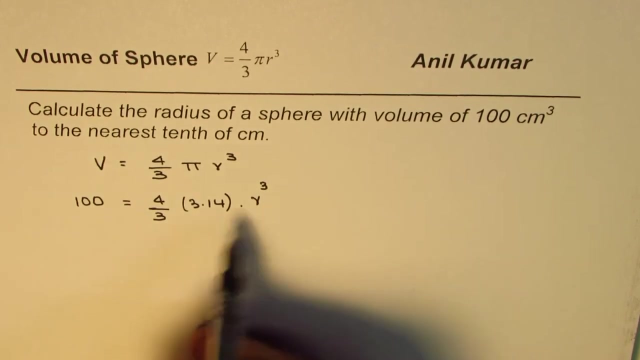 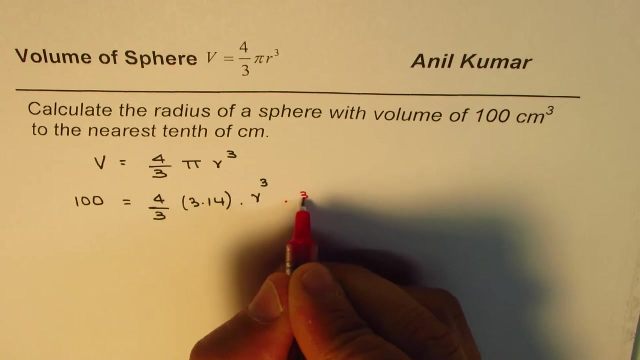 Let me take value of pi as 3.14 for the time being r cube times r cube. So here we know all these values. We need to find the value of radius r To find that we have to do reverse calculations. So to get rid of 4 by 3, we will actually multiply both sides by 3 by 4..